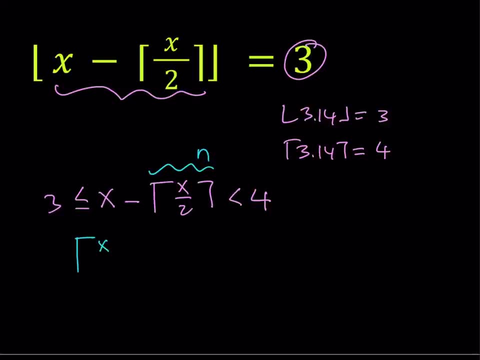 what does that give us? Well, by saying that the ceiling of x over two equals n. you can also use the definition of ceiling, And this means that x over two. now think about a number whose ceiling value is going to be n. Obviously, that needs to be greater than n minus one right, Because anything greater than 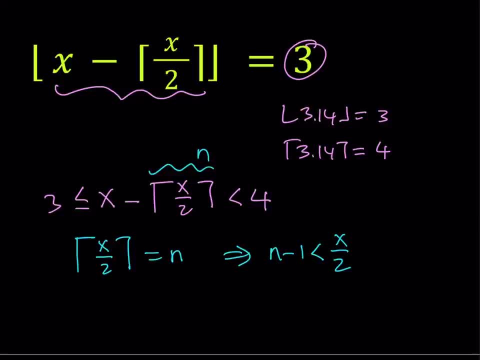 n minus one. if n is an integer, its ceiling value is going to be n, as long as it is less than or equal to n, Because if it exceeds n, then its ceiling value is going to be n plus one or larger. 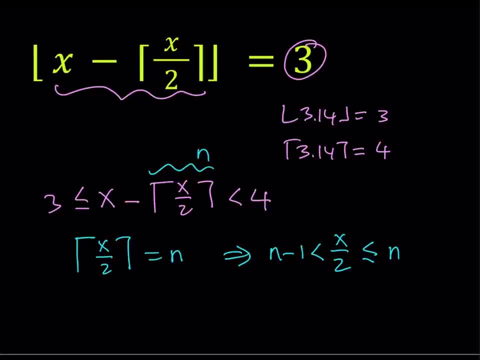 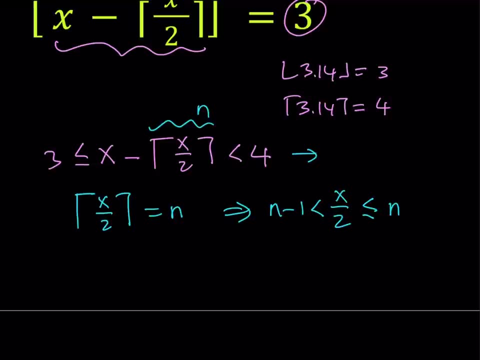 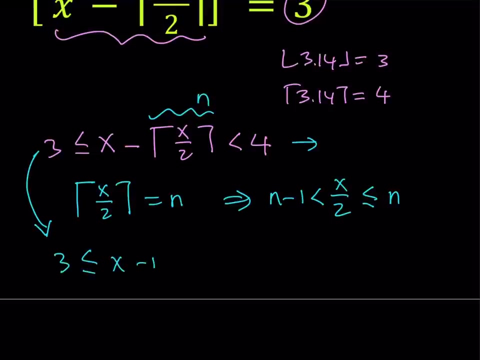 Okay, so from here we're getting this interesting inequality, But we also have another inequality which we didn't write down yet from this one, So let's go ahead and write that down as well and see what that's going to give us. So from here we can say that three is less than or equal to x minus n, and that 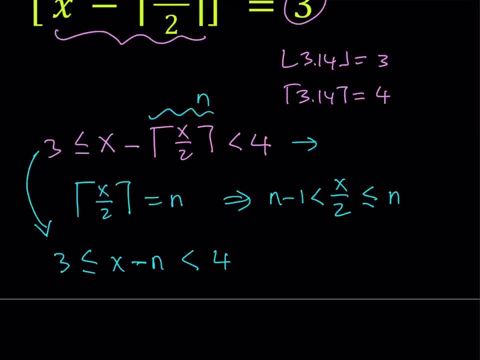 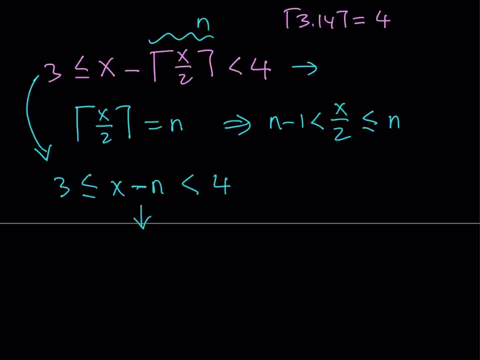 is less than four. So right now I have two inequalities. Hopefully I can solve these inequalities, But let's go ahead, and in each one I would like to isolate x. So add n to both sides by two. I'm good, I'm going to be getting this, And let's go ahead and multiply both sides by two. 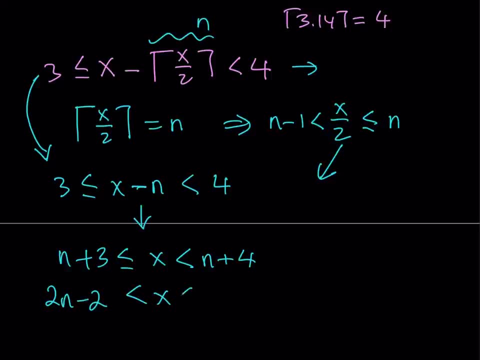 here And we should be getting this one. So I kind of have like a system of inequalities, but I have to be careful because n needs to be an integer in this case. Of course we had to say that at the beginning, but hopefully that you already knew that. So what am I going to do with this system? 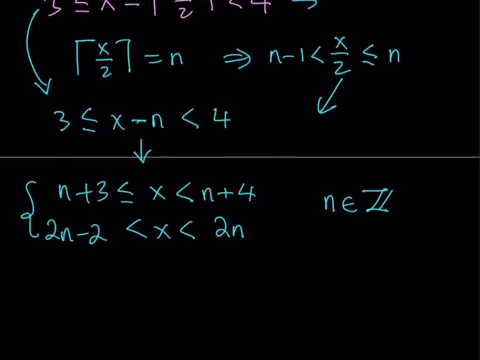 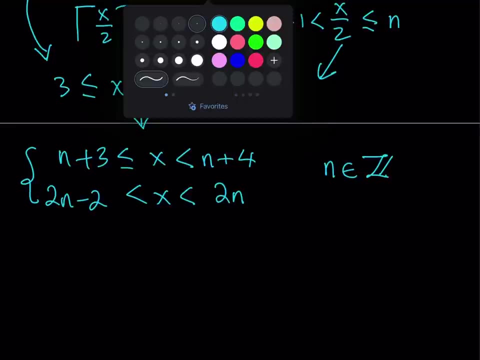 of inequalities. Well, we have to solve it right. How do you solve these kinds of inequalities? Well, first of all, n is an integer and we're looking for x, So notice that this implies something real cool. For example, x is greater. 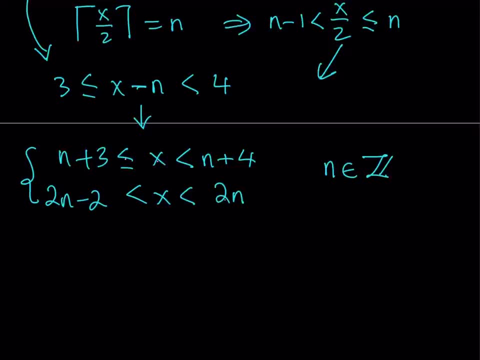 than n plus three and less than two n. So we have like a lower bound here and an upper bound sort of here. That means that the lower bound is always going to be less than the upper bound. So from here we're getting that n is greater than three. That's nice. Let's keep it for now, and then we'll. 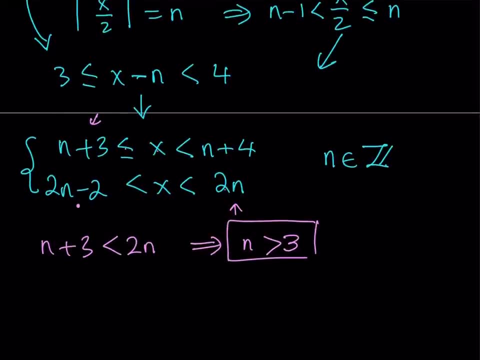 put it together with the other result And we can say the same thing. here We have a lower bound and an upper bound In comparing those. I can say that two n minus two must be less than n plus four, And this implies that n is less than. 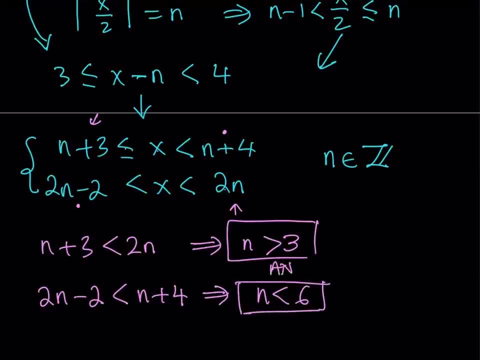 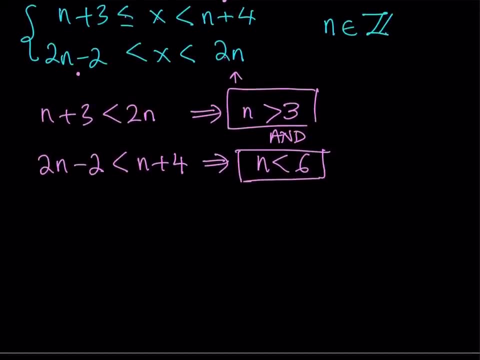 six. Of course, both of these have to happen at the same time, Otherwise we're not going to have this system. So this tells you that n can be four or five, right? So what happens if n is equal to four? Great, Let's take a look. So. 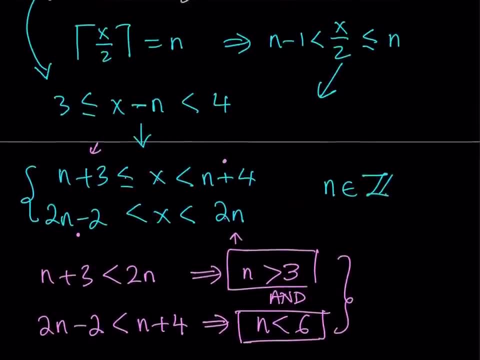 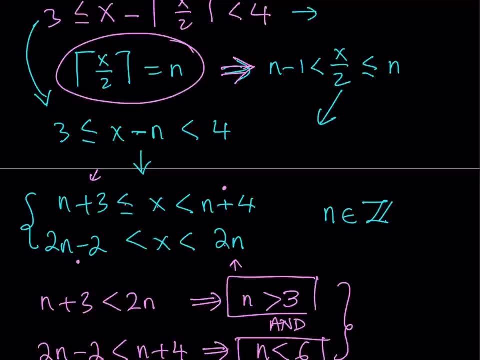 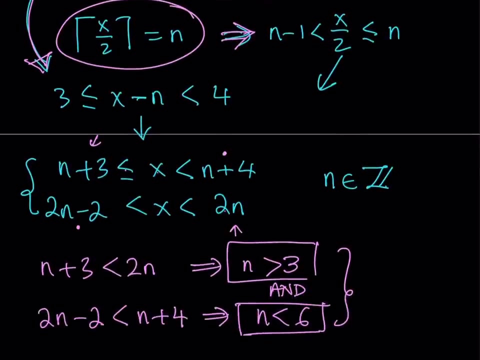 hopefully this made sense. We wrote: you know, by setting this equal to n, we were able to get an inequality like this one by using the definition of the ceiling function, And then from this one we were able to get another inequality. We isolated x in both inequalities and we did. 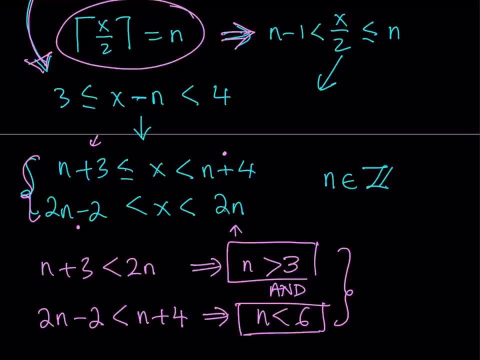 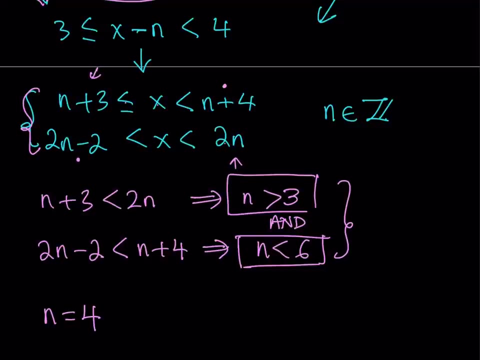 get a system of two inequalities in which n is an integer And we're looking for the x values. Of course, x doesn't have to be an integer, but n has to be an integer And, as a result, we got that n needs to be greater than three and, at the same time, less than six, which implies 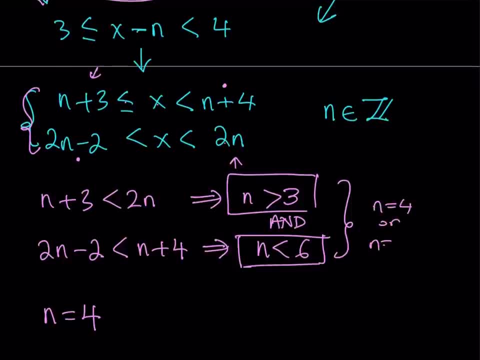 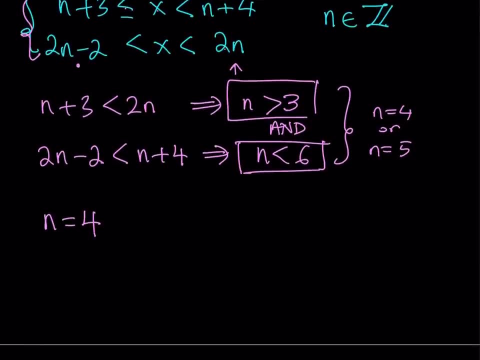 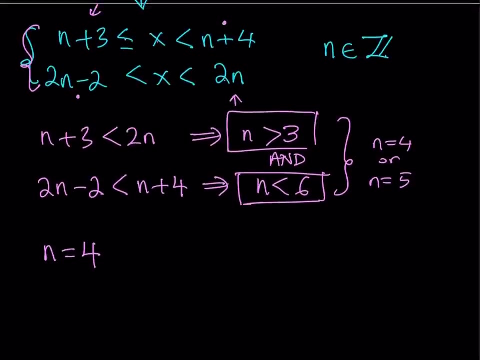 that n is equal to four or n is equal to five. Notice the difference between and and or. There are different things, right, basically? So what happens if n is equal to four? So we're going to look at it case by case. If n is equal to four, we can just go ahead and replace n with four in. 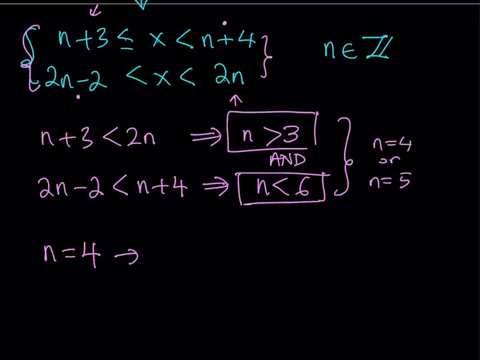 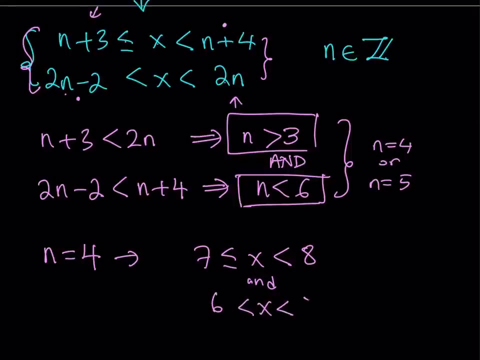 this system. Let's see what happens. This gives us seven, x and eight, And of course there's an n in between them, And when you replace n with four here, that's going to give you six, And two times four is equal to eight. So now you've got a system. 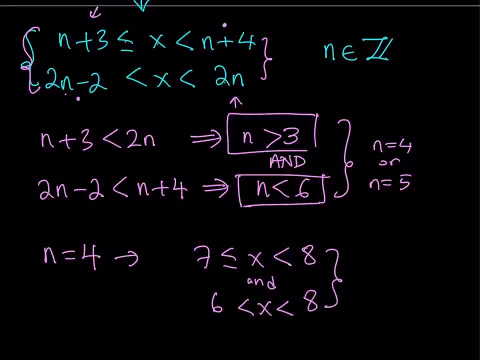 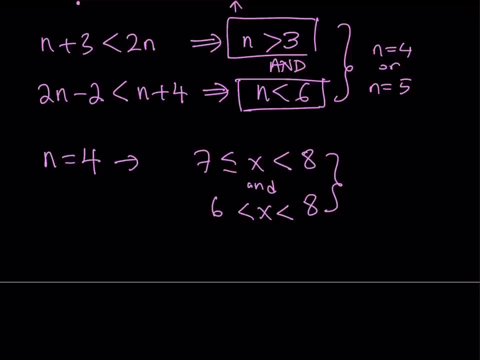 of inequalities again, But this time, instead of having an n in it, it's just numerical value, So you can just go ahead and intersect those inequalities And that's going to give you the interval between seven and eight. Seven is included because 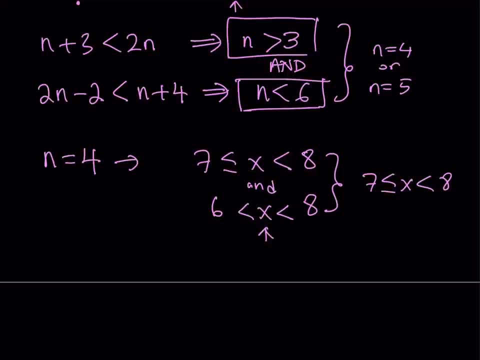 seven is between six and eight, but eight is not included because none of these equalities or both of these inequalities don't give me eight. So that's going to be part of the solution, And then we're just going to put it together at the end, okay, So let's go ahead and take a look at the 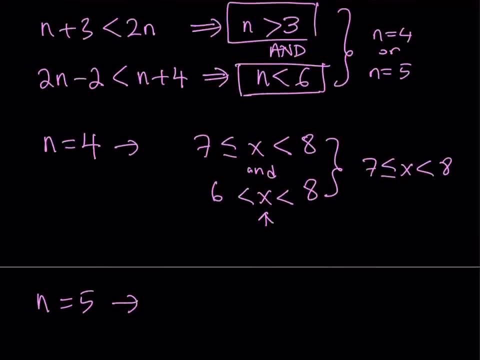 case where n equals five And you do the same replacements pretty much, If you do. well, for n equals five, you're going to be getting something like eight is you know x is between eight and ten and between eight and nine. Of course we're going to be getting something like eight, is you?